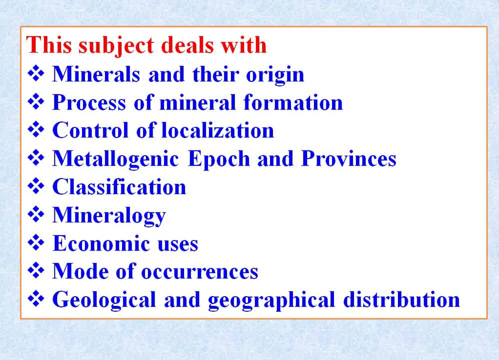 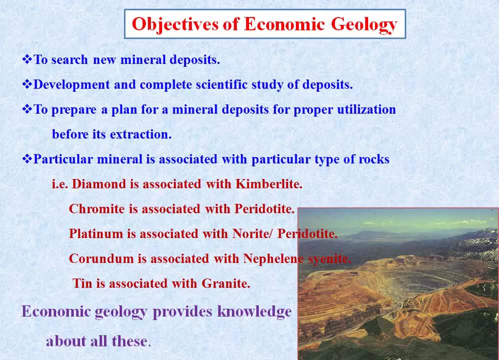 Economic Geology: economic uses, mode of occurrence, geological and geographical distribution. Objective of the Economic Geology: The main and important objective of Economic Geology is to charge new mineral deposits. The main and important objective of Economic Geology is to charge new mineral deposits. 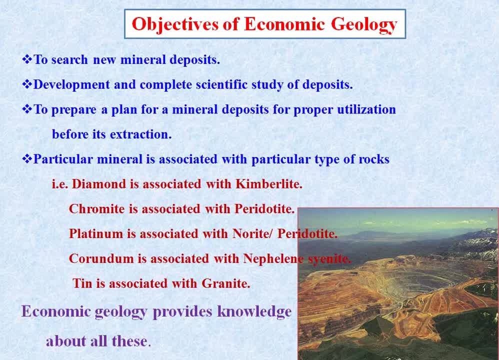 The main and important objective of Economic Geology is to charge new mineral deposits, The development and complete scientific studies of deposits. The development and complete scientific studies of deposits. To prepare the plan for a mineral deposit for proper deficits. To prepare the plan for a mineral deposit for proper uses of mineral deposits. 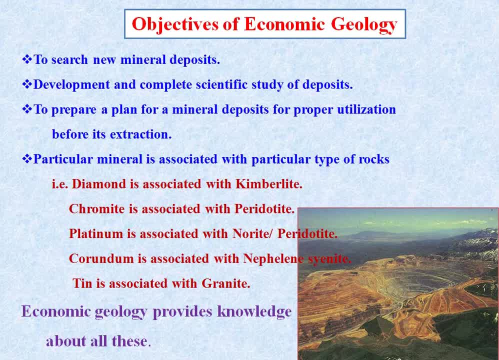 a particular mineral in nature is associated with particular types of rocks. for example, diamond is associated with kimberlite. chromite is associated with peridotite. platinum is associated with norite or peridotite. corundum is associated with naphthalene, cyanide, tin. 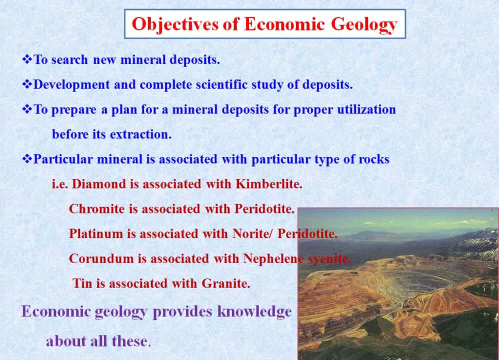 is associated with granite. hence we can say that there is a genetic relationship of minerals with the particular types of rocks. so economic geology provide this knowledge about that, that a particular rock is host a particular types of minerals. so economic geologists have an idea about the assemblies of mineral in a particular types of rocks. so economic 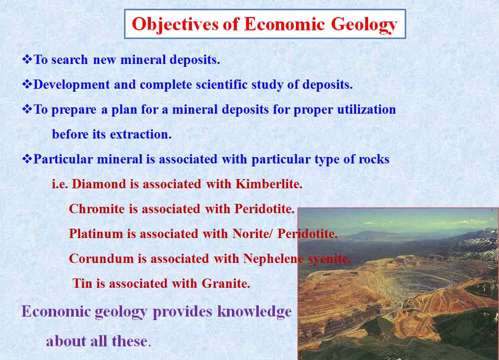 Geology provide the detailed knowledge about it. In nature, a special type of mineral is associated with a particular type of rock, such as diamonds are always found in the kimberlite. in the same way, chromite is associated with peridotite. 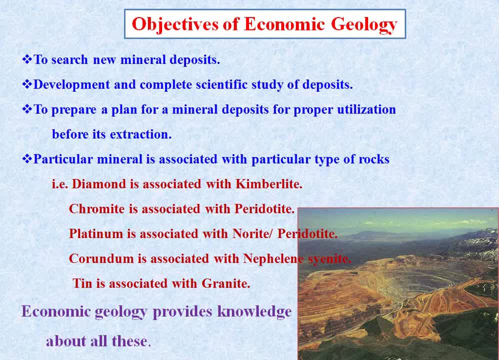 in the same way, platinum is found with norite or peridotite, corundum is found with nephelinsinite and tin is found with granite. In this way you can say that rock has a genetic relationship with mineral association. So all this knowledge provides us with economic knowledge. 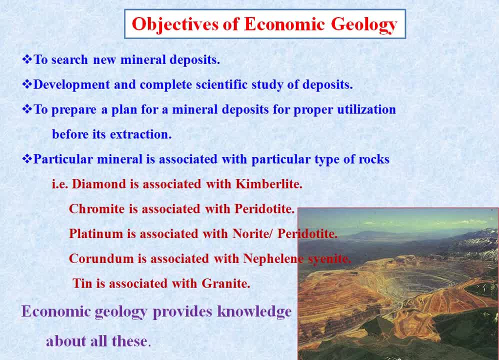 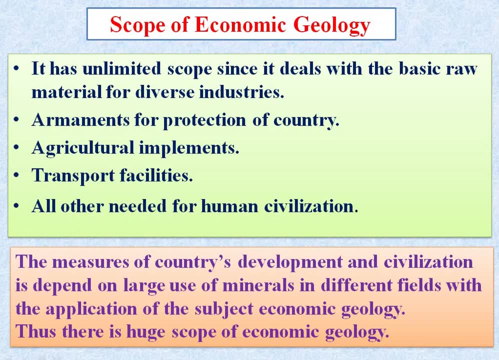 Due to which it is easy for us to search for new minerals. Scope of economic geology: the field of economic knowledge. the field of economic knowledge is a long and wide field. Yes, divers and weak. open casket name. so yeah, basically say so, be good, you know. 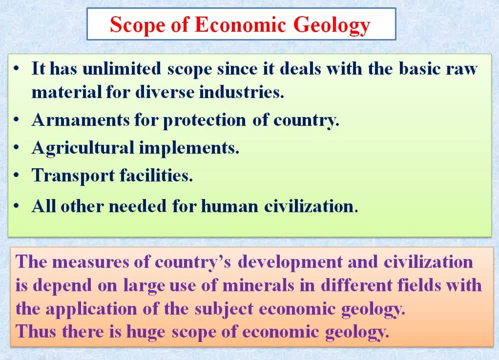 kachamal provide. karate is yellow, a desky raksha kill you. so us, the sister, went ahead. agricultural implements are carciga up, Garan, household utensil, all transport facilities and all other things need for human civilization. mano sabita, kill you to be our sector of the economic geology will. 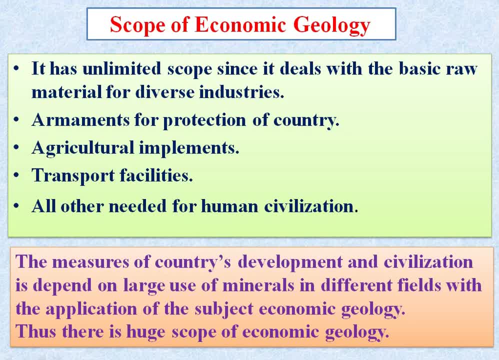 upload the Carvata a kissy days carthaginous. this key can is some. panama never got time for honey. somebody got it not use with. I do you do, Sarah? knowledge, a economic geology, provide Carvata a test. there is a huge scope of economic geology. 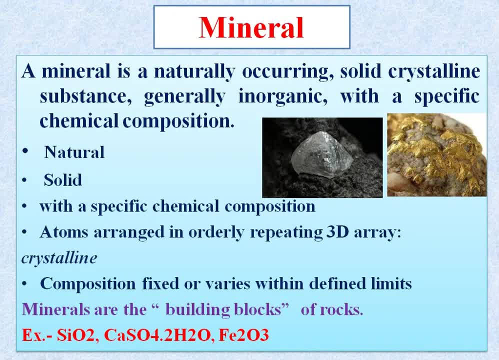 now we discussed the mineral. what is the mineral? a mineral is naturally occurring solid crystalline substance, generally inorganic, with a specific chemical composition, human, natural otahe, solid with a specific chemical composition, atom arranged in a orderly repeating three-day array and crystalline and composition is fixed. so minerals are. 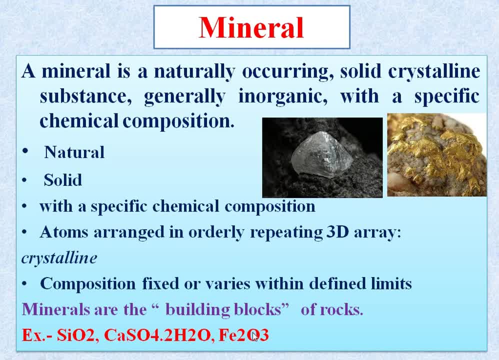 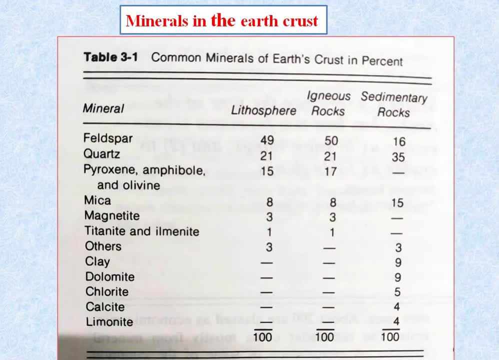 building blocks of the rock, for example quad, gypsum, hematite, at sector minerals in the earth crust. so this is the common mineral in the earth crust in the percentage. for example, failspare compose the 49 percent of the Lithos fear, and then followed by the quads 21%. the pyros in amphibole and oliving compose 15. 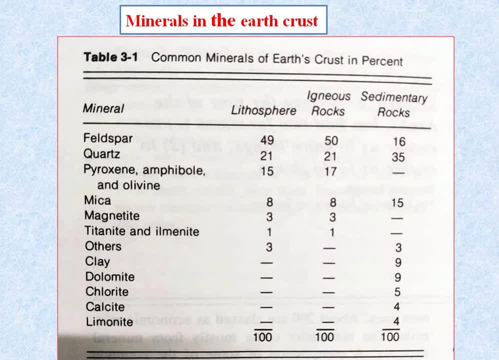 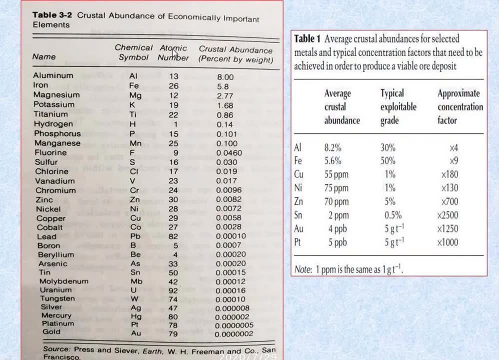 percentage, then other, followed by mica, magnetite, titanite, illuminate and others. this is the crystal abundance of economic important minerals in which oxygen is the most abundant element, then followed by silica, then the alumina in the eight percentage: iron 5.8, magnesia 2.77, potassium 1.68, then titanium. 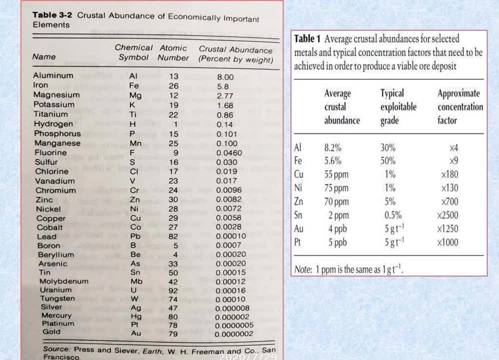 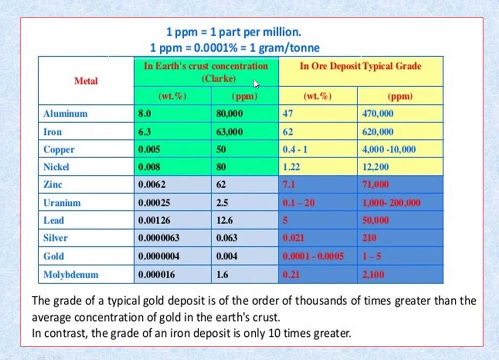 hydrogen phosphorus, manganese, fluorine and gold in the last, so the element which have very least concentration. these are very precious minerals. this is also a earth crust come. concentrations are chart given by color in this: aluminum: aluminum: eight. percentage. iron: six point three percentage. copper: zero point zero, zero, five percent. nickel: zero, zero point eight. 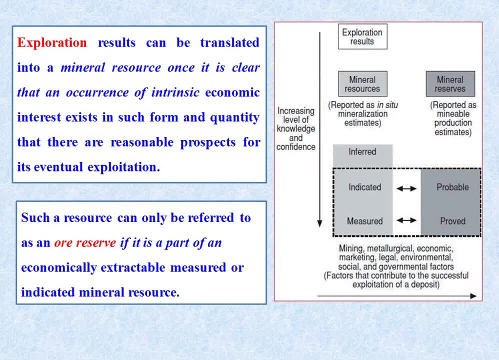 now the exploration. exploration results can be translated into mineral resource once it clear that occurrence of intrinsic economic interest in such form and quantity that there is reasonable prospect for its eventual exploitation. such a source can be referred to an ore deposit if it is a part of an economically extractable. 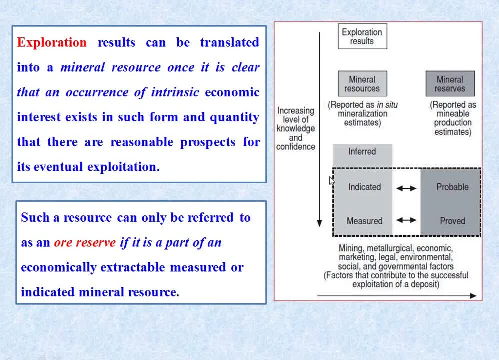 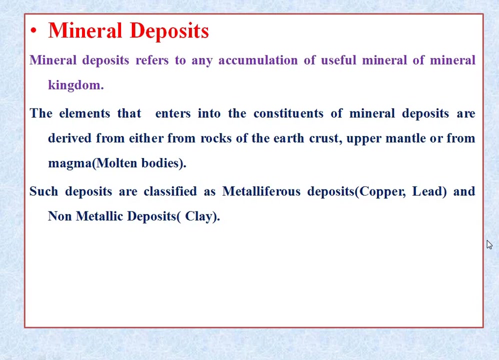 measures or indicated mineral resources. mineral resources and mineral reserve resources are in-situ estimates and reserve which are reported as mineable production in which there is a chart. mineral resource may be inferred, then indicated and measured so and reserves are probable and proven, proved. now, mineral deposit: mineral deposit refers to accumulation of useful mineral of. 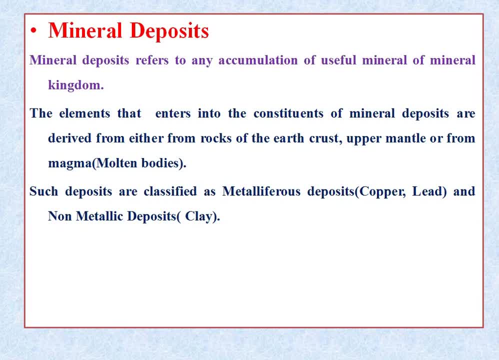 The mineral kingdom. The shape of the well. The same type of well is in one place. It is called the shape of the well. The elements that enter into the constant trend of mineral deposits are derived from either rocks of the earth, crust, upper mantle or from magma, The minerals that are together. 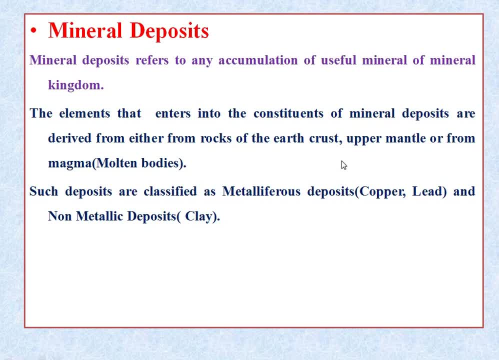 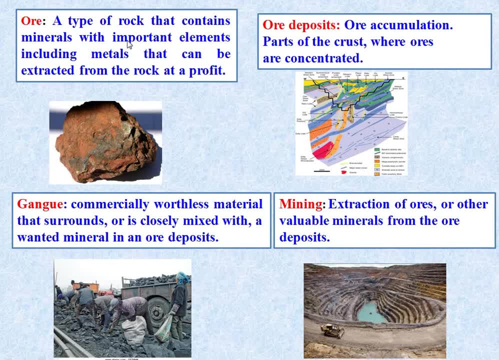 Now there are some terminology regarding economic geology, or or a type of rock that contains minerals with important elements, including metal, that can be extracted from a rock at a profit. Yes, What is ice called? Any rock can be extracted from a rock at a lab. It is called ice. 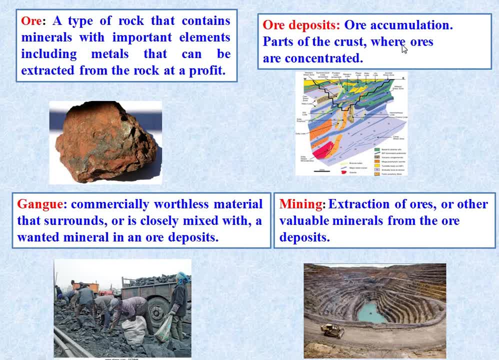 Ore deposit: Accumulation of ore from crust where ores are concentrated. Now gang or Adatari is called. This is unwanted associate of the ore, Along with ice, some acids are added to the ore and they are called gang. Commercially worthless material that surround or closely mixed with a. 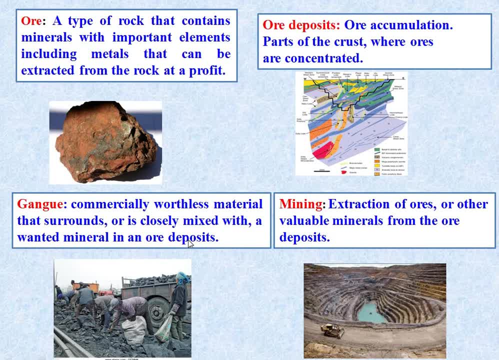 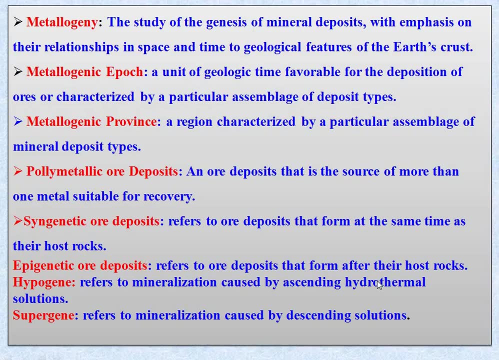 wanted mineral is called ore deposit. Adatari or gang is called Now the mining. The extraction of ore or other valuable mineral from the ore deposit is called mining. mining is called mining. mining is called mining. Now some terminology related to the economic, geology, metallogenic. 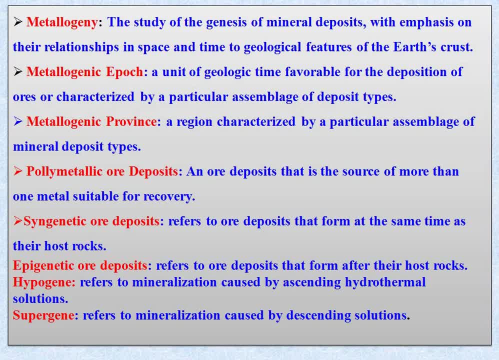 to study of genesis of mineral deposits, with emphasis on the relationship in space and time to geological features of the earth crust. What is metallogenic? How did the emergence of the Kheniz snake shape occur? Along with that time and time and space, the study of geological features? 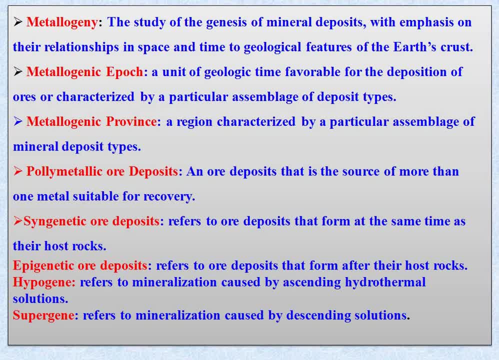 is called metallogenic. The study of geological features is called metallogenic. Now, metallogenic epochs: A unit of geological type favorable for the deposition of ore characterized by a particular assemblage of deposits, The time of geological history which is appropriate for mineral deposits. 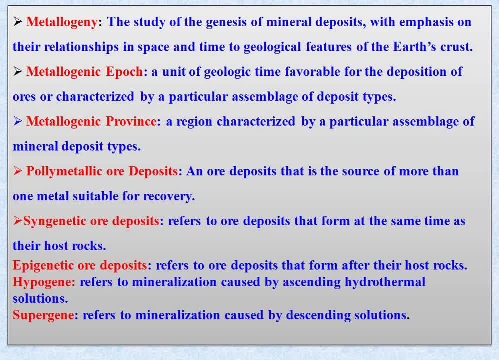 metallogenic epochs, For example, Pre-Cambrian epoch metallogenic province, a region characterized by particular assemblage of mineral deposits. A region characterized by particular assemblage of mineral deposits, an area which is suitable for special type of Kheniz snake shape. 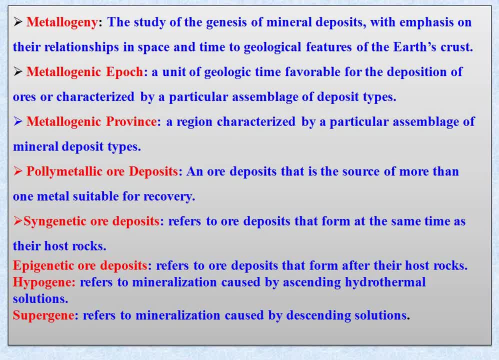 is suitable for metallogenic province, For example Aravali province. Polymetallic deposit is a deposit in which more than one mineral is found, which is called a polymetallic mineral, such as gelcopyrite, in which copper, iron and sulphur are found. 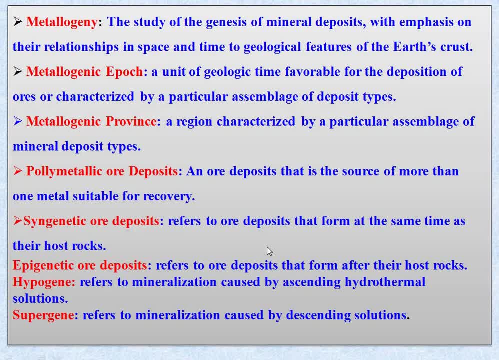 Syngenetic ore deposit is such an ore deposit that is made with the host rock. Epigenetic ore deposit is such an ore deposit that is made after the host rock. Hypozine is a repulsive mineralization caused by ascending hydrothermal solution. 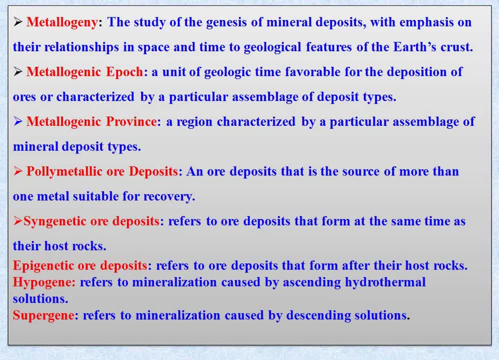 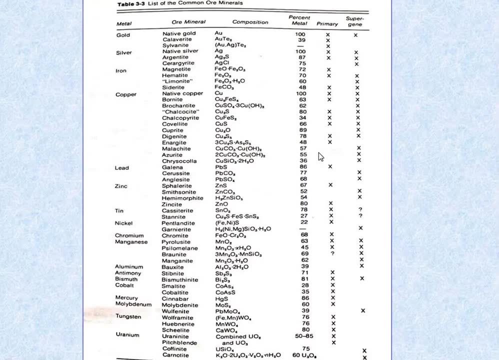 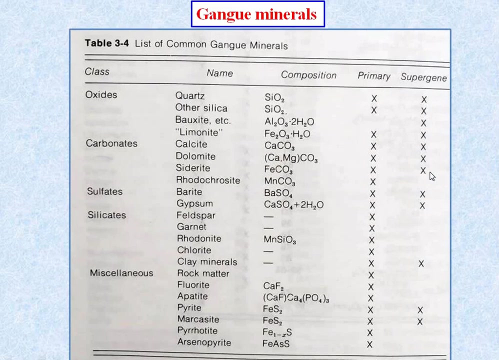 Hydrothermal solution in which later ascending is called hypozine mineral deposit And now superzine. These are secondary mineral deposits which are mineralization caused by descending solutions. This is the list of common ore minerals. These are the list of common gang minerals. 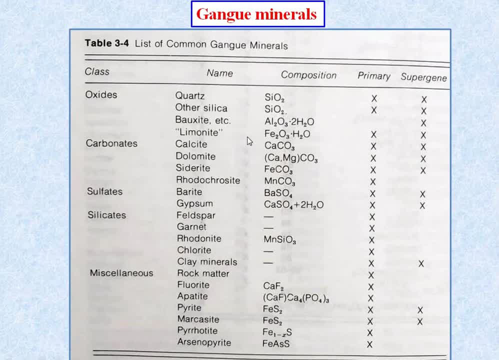 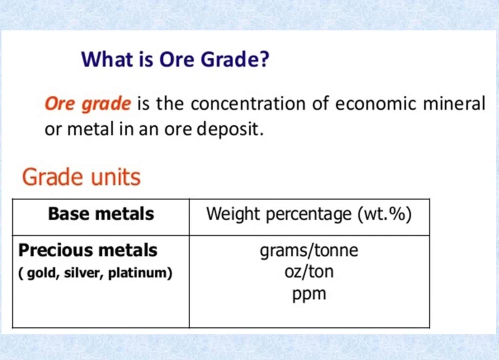 Commonly gang minerals are quartz, limonite, calcite, dolerite, barite and etc. Now what is the grade? Grade is the metal content of an ore. In any ore, the higher the percentage of metal, the better its grade. 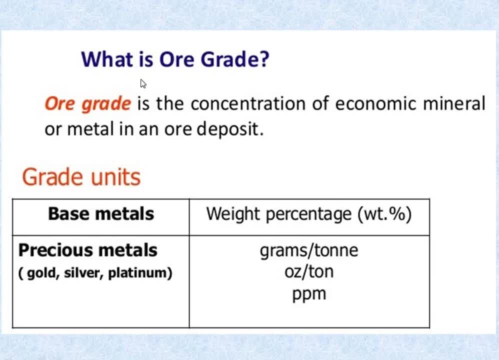 The higher the percentage of metal, the better its grade. The over grade is the concentration of economic, mineral or metal in the ore deposit. If it is base metal, generally, we write its unit in the weight percentage, and if it is precious metal, then we write it in gram per ton.